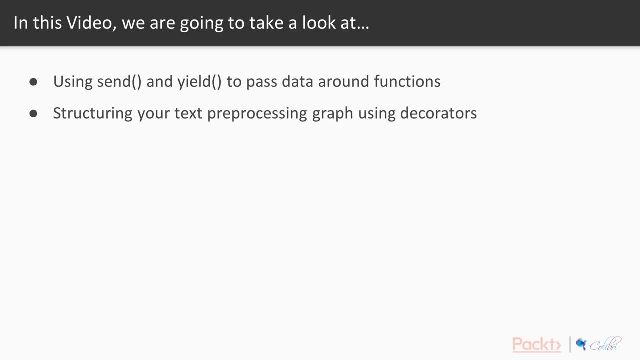 You always have to go one input into a model, one output, and you take that output into another model, Meaning that you cannot Take the outputs of one step and feed it into two different models with two different outputs and then maybe either combine them or discard one of them and then use the other one. 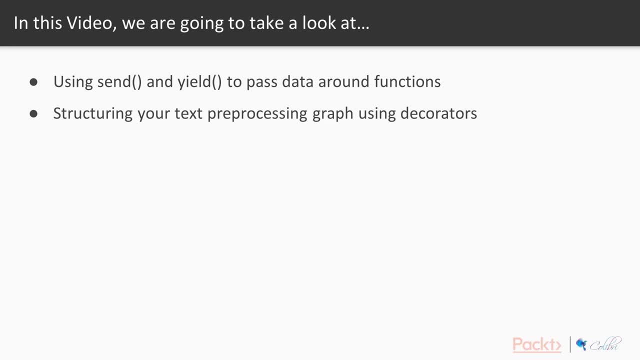 You can't do that right. Furthermore, it's also sometimes hard to combine NLTK and scikit-learn functions, And NLTK is obviously purpose designed for natural language processing, So we want to use it as much as possible. So I'm going to show you today what are the NLTK functions that is commonly used to pre-process. 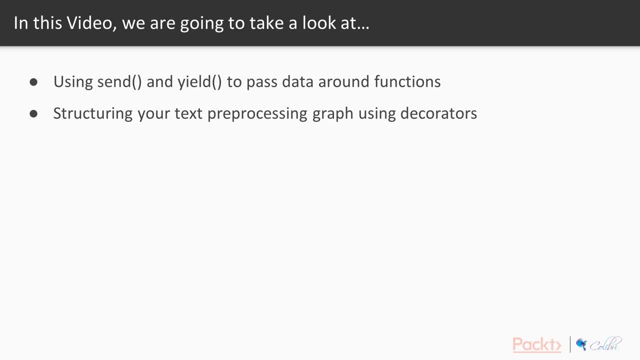 Okay. So first of all, we're going to show you how we can use natural language to make it structured language data so that it's ready to be vectorized and fed into machine learning pipelines. Number two: how we can use the send and use generators in Python standard library to create 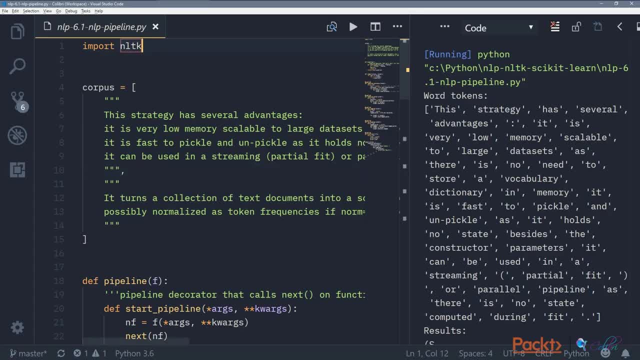 a data or a text pre-processing graph. Let's get right to it. So, some housekeeping. we're going to import NLTK, unsurprisingly, and we're also going to set a corpus. This corpus is simply A few sentences. 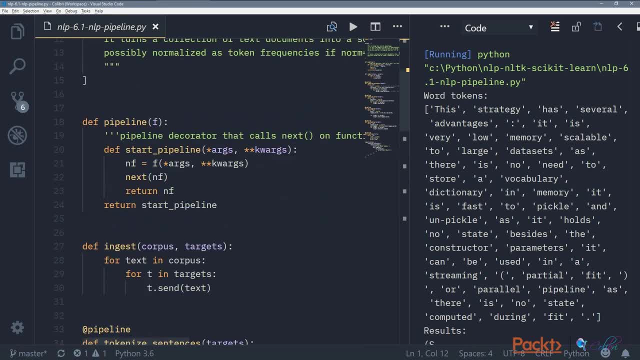 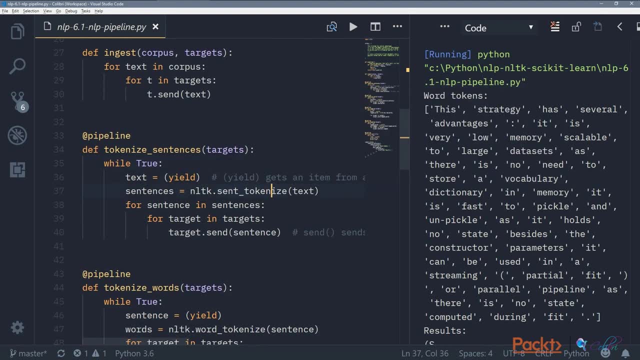 It's just A lot of text. So if you want to use the 솥 to create this corpus, you'll need the text pre-processing graph to do it. So here is what we want to do. All right, We're going to go over the NLTK functions that are commonly used for text pre-processing. 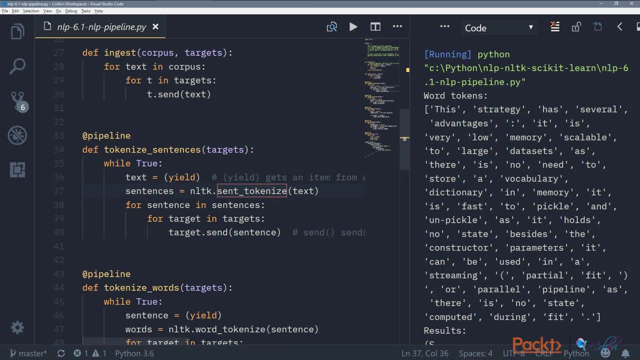 So they're sent tokenize, which splits a text into sentences, And while this might seem very intuitive- actually, because let's say, ellipsis is three footsteps and then you have to distinguish it's between that's at one footstep And also what happens- 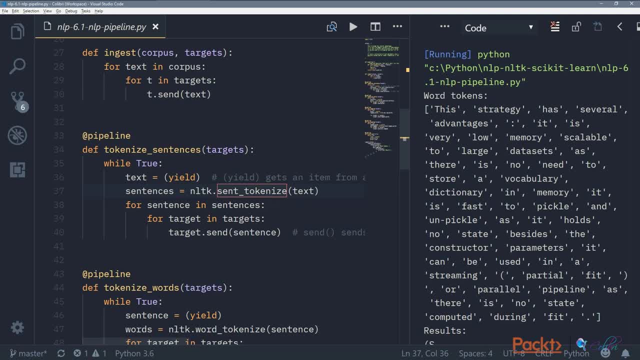 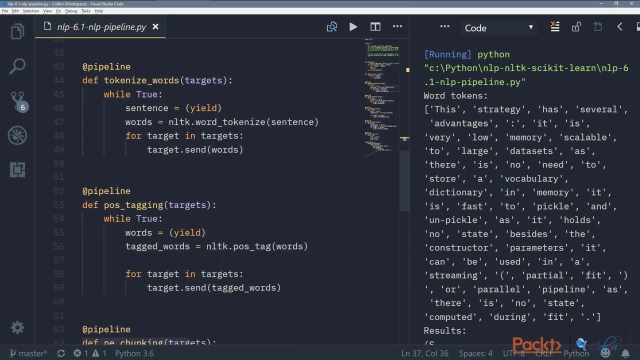 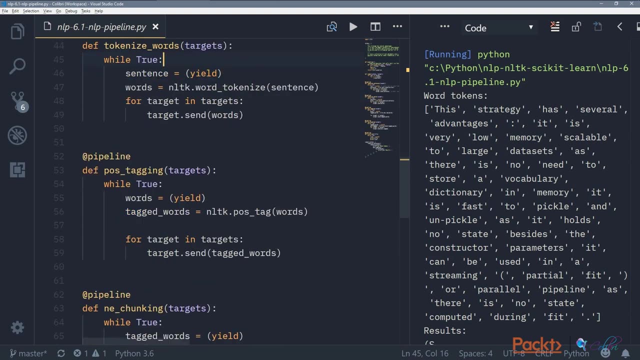 how do you take care of parentheses, etc. so sent tokenized contains all these rules and you can just deploy it and it would nicely separate it into sentences and a word tokenized we're very familiar with, we. this breaks up a sentence into words easy. POS tagging stands for parts of speech tagging, so what this does is 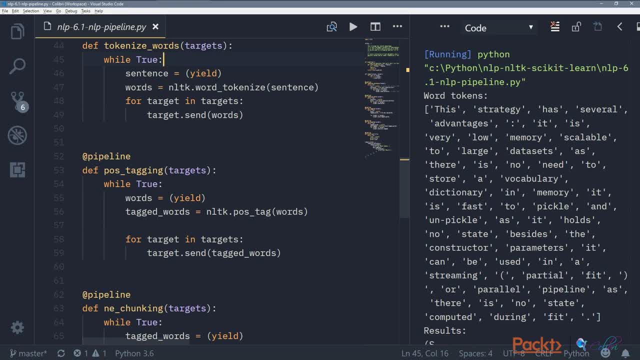 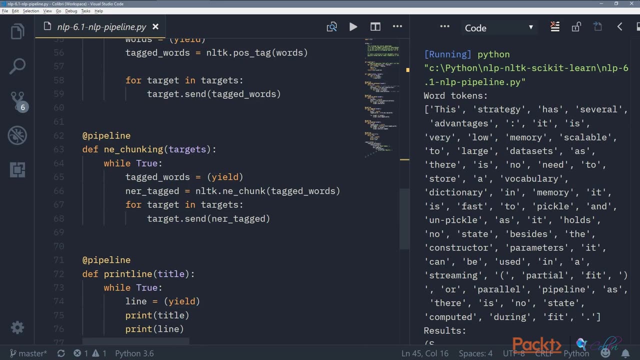 it tags words in whether it's a noun or adverb, so these position tags can be used to inform downstream models about what this word is and help on inference. and then any chunking is trying to extract noun phrases, so it's a little bit like two grams and three grams, but instead of blindly taking two words. 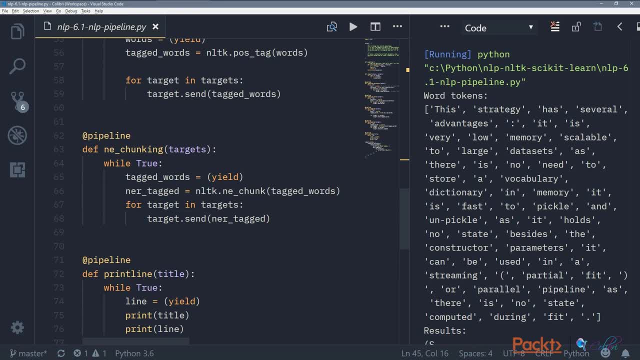 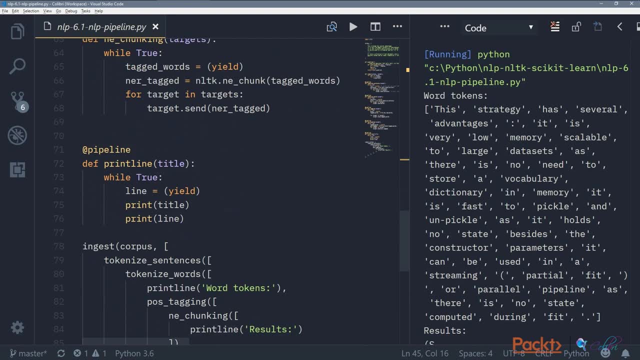 that's, you know, come after the other, or three words that come out to the other. any chunking tries to intelligently extract phrases that make sense, given what the word, given the corpus. so how do we create this problem? So how do we create this problem? 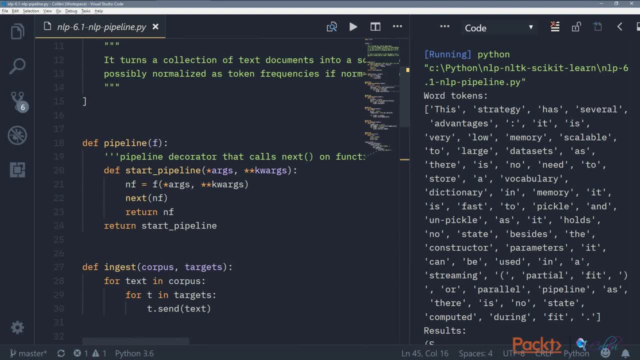 So we first need a pipeline decorator which takes in a function f. in that pipeline decorator we have a defined inner function called start pipeline which just simply passes on the arguments and the keyword arguments. we first call and assign the function with the arguments into new function and it 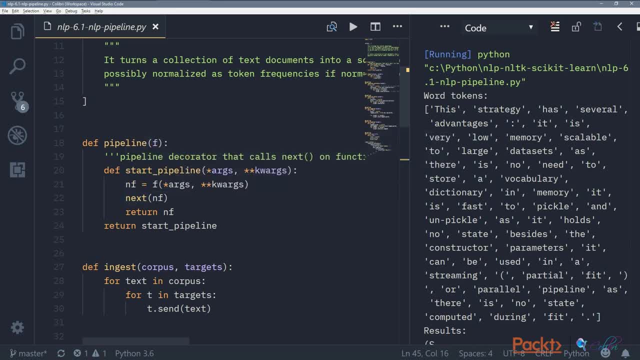 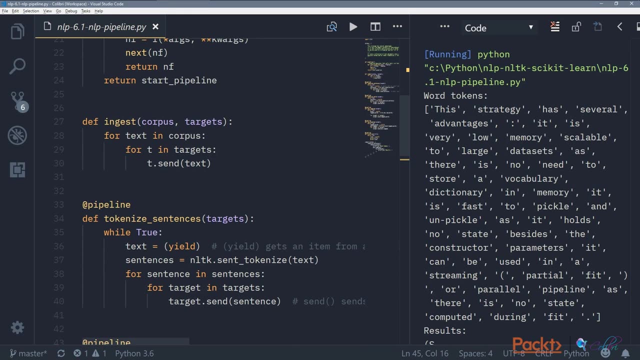 would call next on the function. so doing this allows us to feed in a function that is generator, and calling next allows it to then feed data through. so there are two key words we remember here. so number one is send, which sends data into the targets and in the target functions we can use. 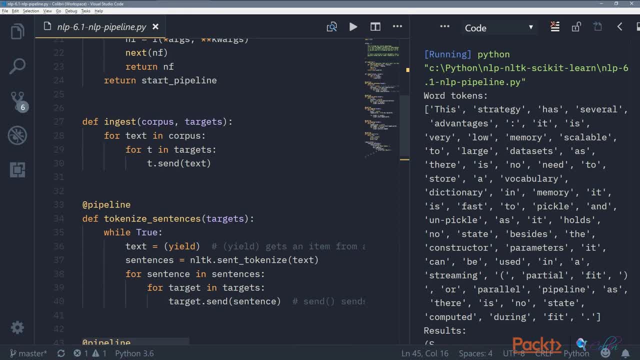 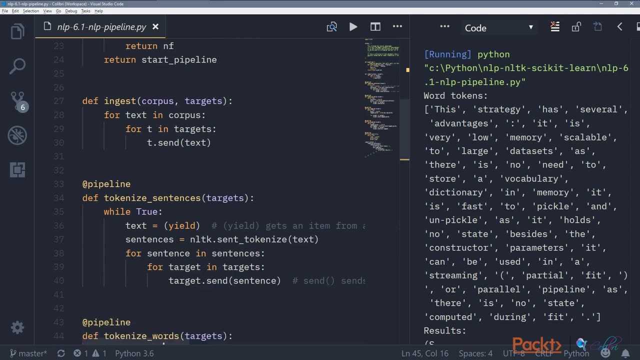 the yield keyword to get back to data from sent. so what this allows us to do is to then pass data from one stage to another and also pass the data to all the targets instead of just one target like what we have in scikit-learn. so if we wrap all of the NLT, 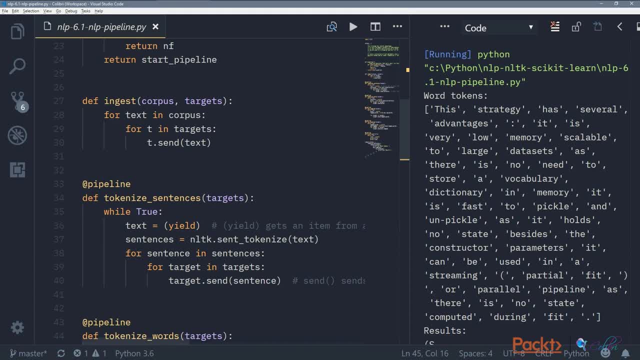 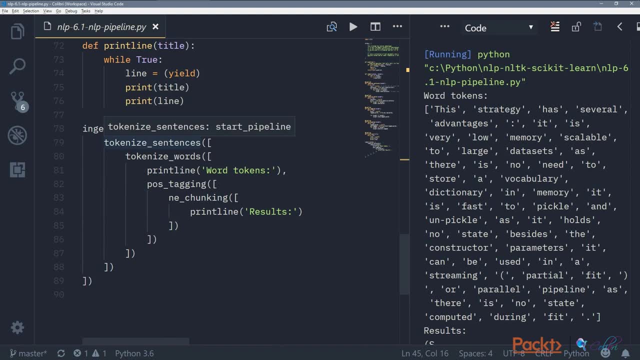 steps with function like this and use the pipeline decorator. we can then create a text preprocessing graph like this one, where we have ingest tokenized sentences, tokenized words, and then put like an or pipe the outputs of tokenized words into two different stages, where we one first print it and then we then pass. 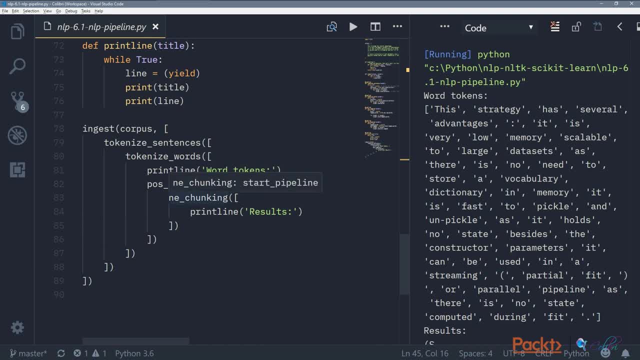 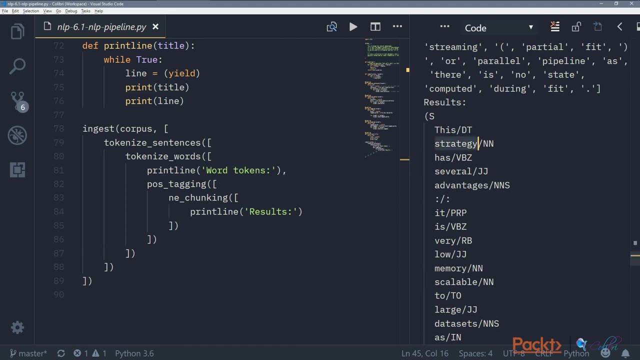 it further on to parts of speech tagging and an any chunking and then print it again. we run this. we can see that after splitting it into sentences and words, we then print it and then feed the rest of results into parts of speech tagging, which is what happened here. so, for example, strategy is a noun and it is a. 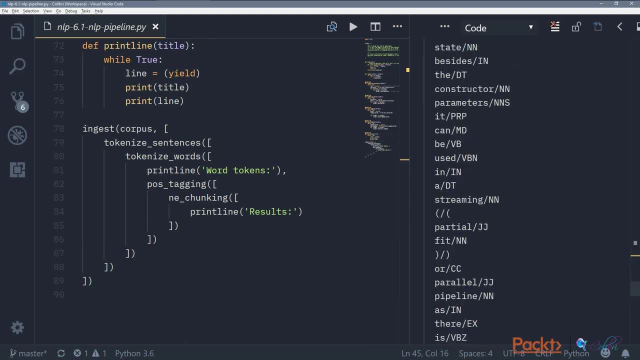 proposition, and then we also have chunked the nouns, so we have things like: scipyparse is a chunk noun, or we can have parentheses here with or binary occurrence information, and that's all there is to it. So we've just learned how to use the generating functions send and yield in.